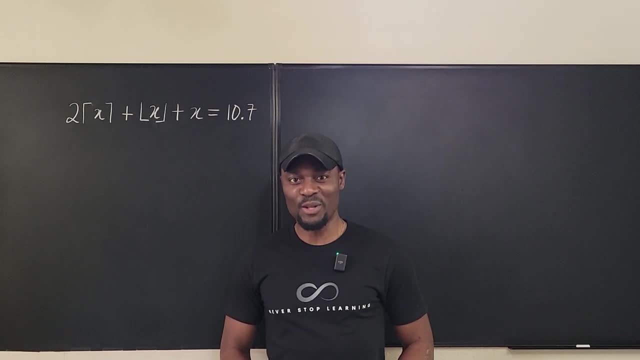 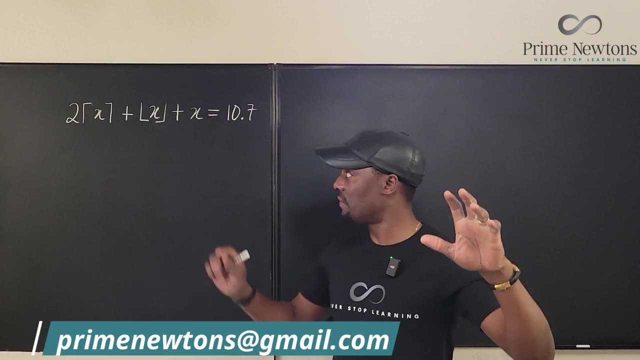 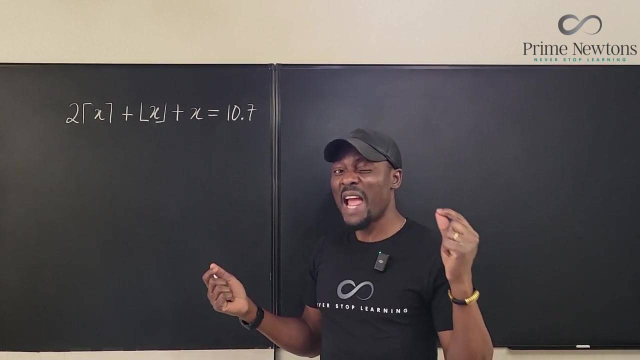 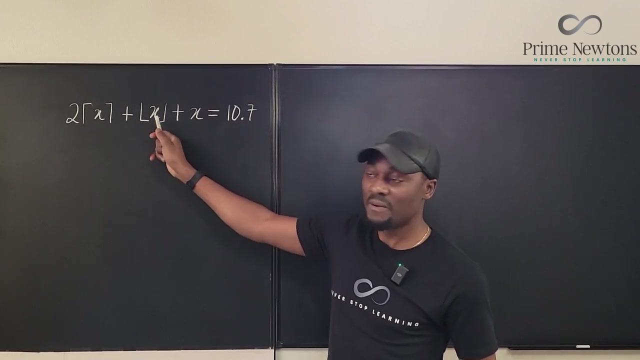 Welcome to another video. This is an equation combining the ceiling function with the floor function, with just a regular function, And we're supposed to find what x is. Remember, we're looking for this guy inside, The guy under the ceiling, on the floor, outside, on the street and everything. 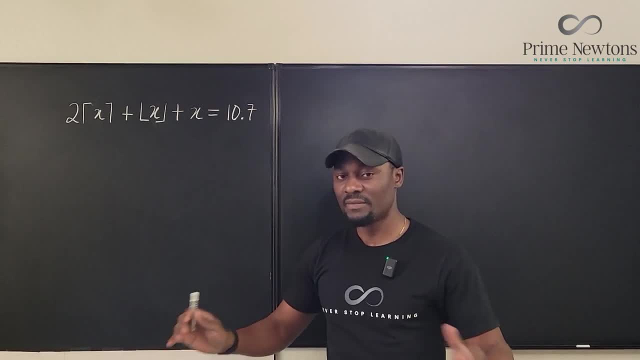 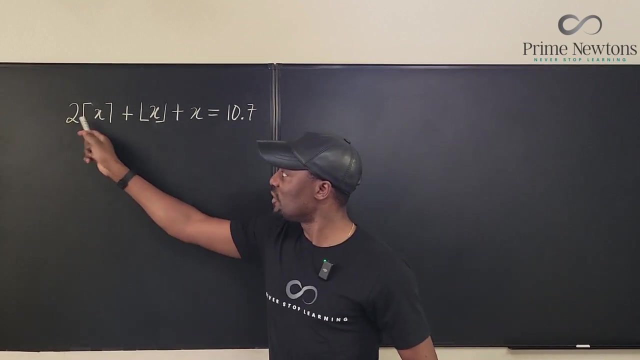 added together is going to be 10.7.. This is going to be super easy And because I want to use this to explain the concept, I decided to choose the simplest form that you can get. It becomes more complicated when you move this two inside or when you start squaring the entire thing. then it 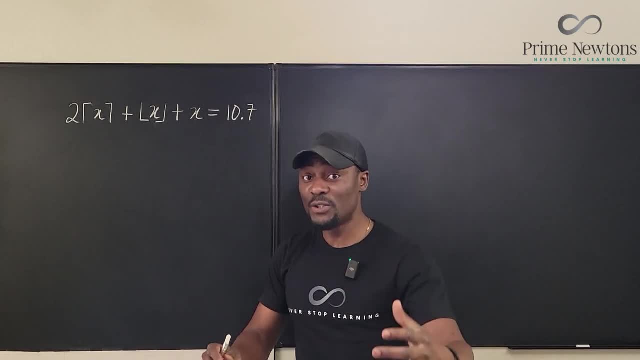 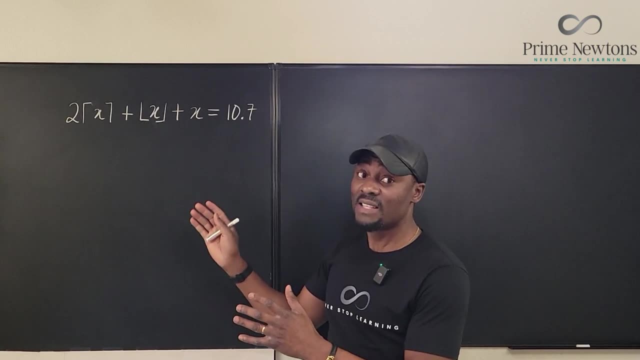 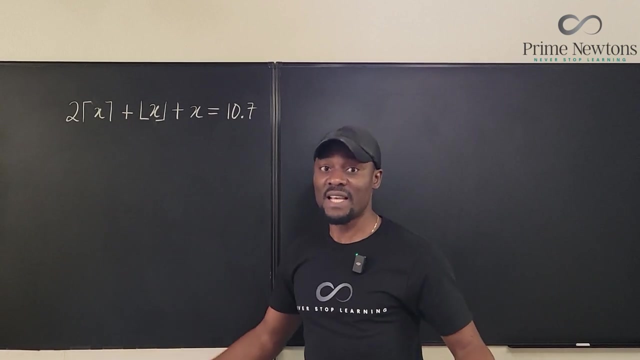 becomes crazier, Okay, But in order to know how to solve this when it gets more complicated, we'll solve this simple one, Okay, And you can even look at this and guess the answer. If you just take your time and guess, you'll get the answer correctly. But in case you don't like guessing, 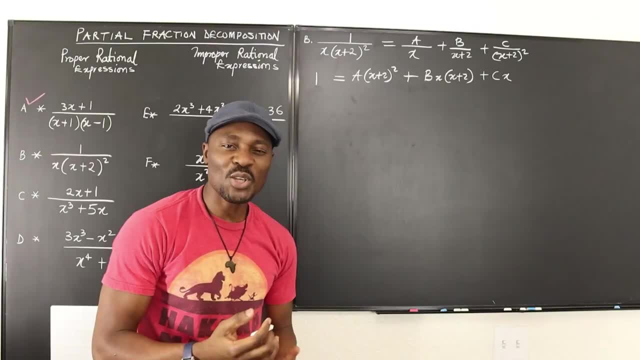 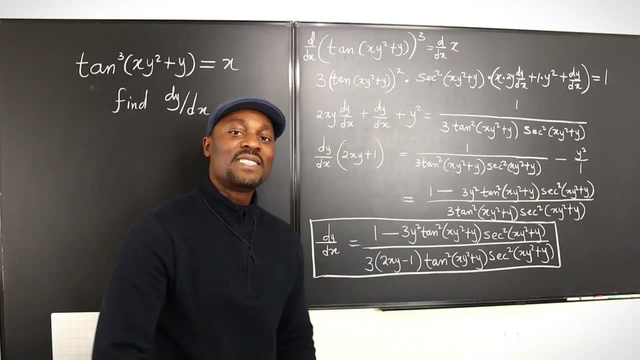 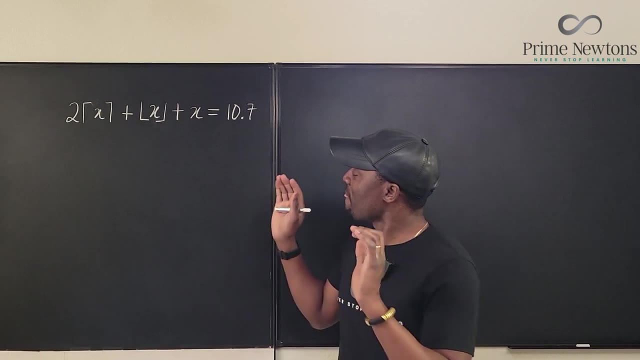 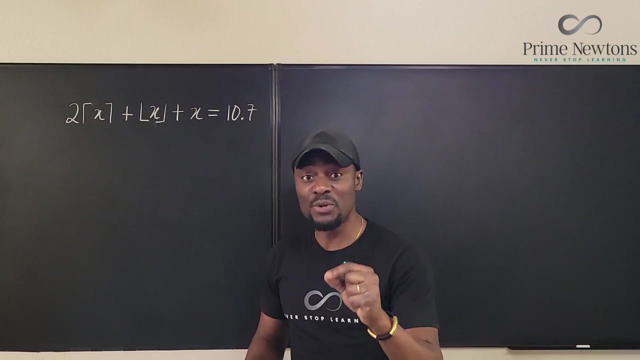 like me, let's just get into the video. So we're going to start by just looking at what typically happens when you do this. So we're going to start by just looking at what typically any number is written as, Remember, it doesn't matter what the number is, Any number. 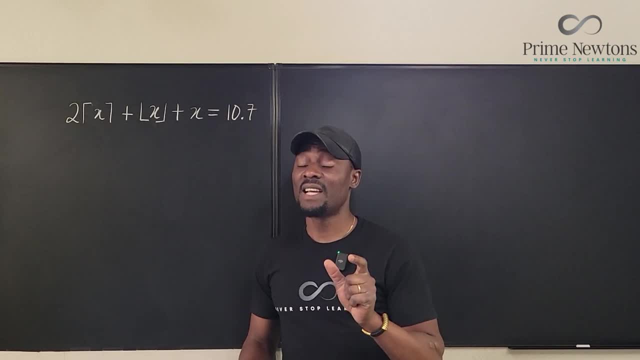 you write has an integer part and has a decimal part. Now, sometimes the integer part is zero and sometimes the decimal part is zero. Every number you write has an integer part and has a decimal part. So every X you write. So note: 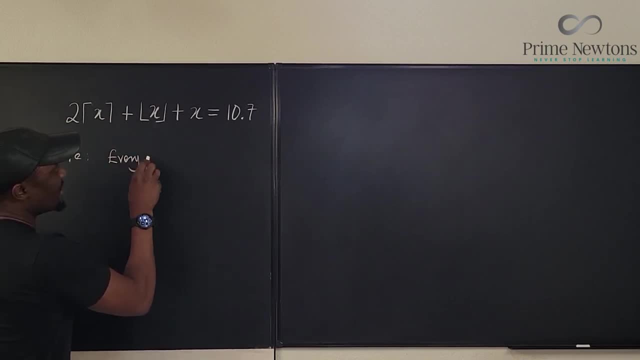 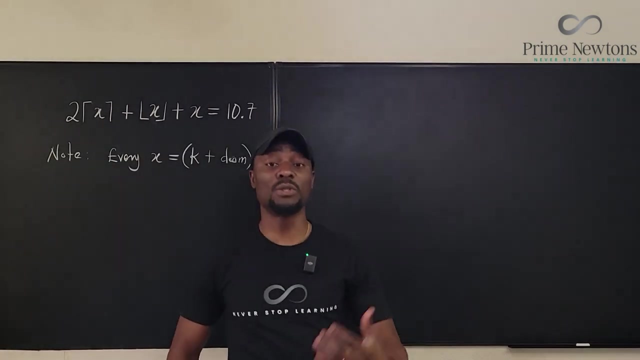 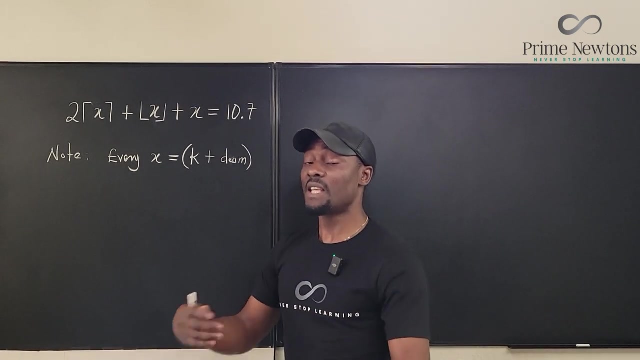 that every X is equal to K plus a decimal. I'm going to write it as decim. Okay, this is every number you write. So let's say you write the number two, It is two plus a zero decimal. If you write the number seven point five, it is seven plus zero point five. 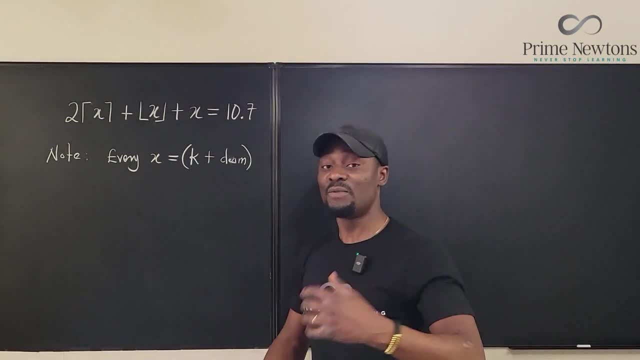 There's always an integer part and a decimal part. If you write 0.5, the integer is 0 and the decimal is 0.5.. That's how you do it. So if you look at the problem that we have, 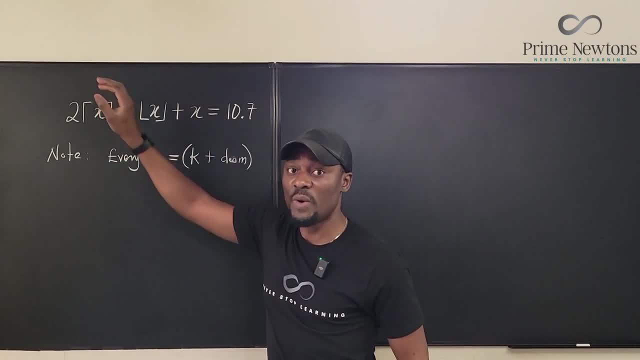 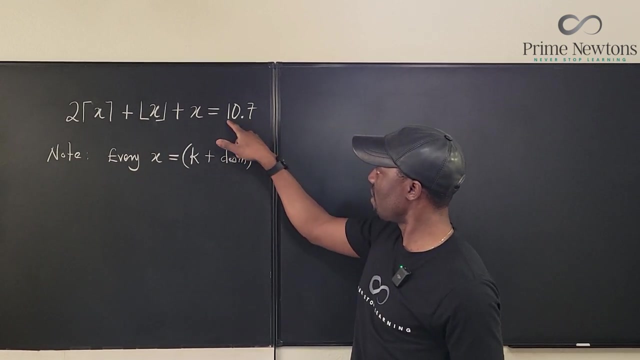 whatever comes out of a ceiling function is always an integer. Remember, by definition, the ceiling of x is the smallest integer greater than x. So if this was, for example, the ceiling of this number is going to be 11 and the floor of this number is going to be 10.. 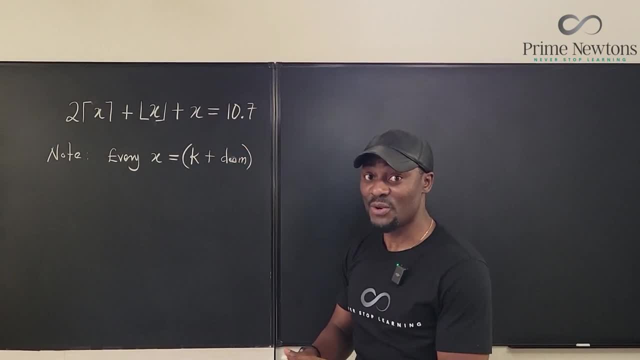 So this has given away. this example I just gave tells you that this is always the floor of x, And if you want to get the ceiling of x, you just need to add 1 to this, because then you go to the next number. 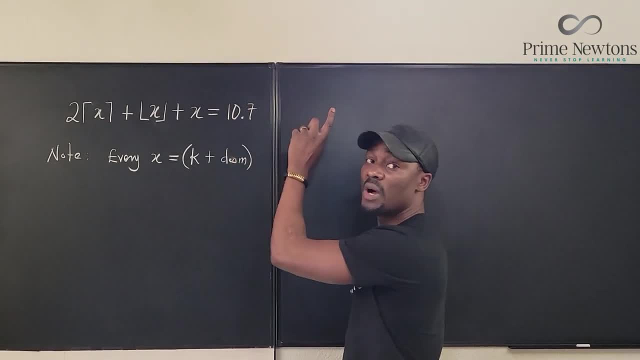 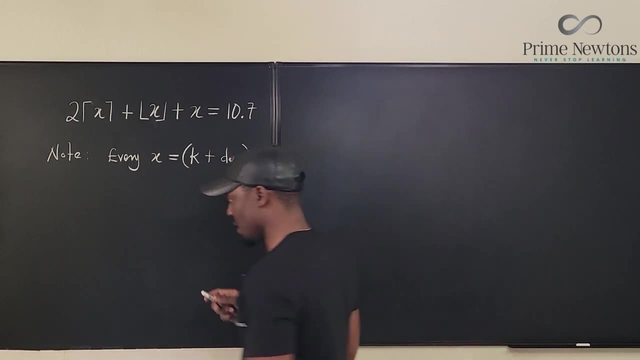 So the ceiling of 10.7 is 10 plus 1.. So the decimal part is converted into a whole number and the ceiling of 10.7 is 10 plus 1.. And you add it to the floor. Okay, so we can say generally: 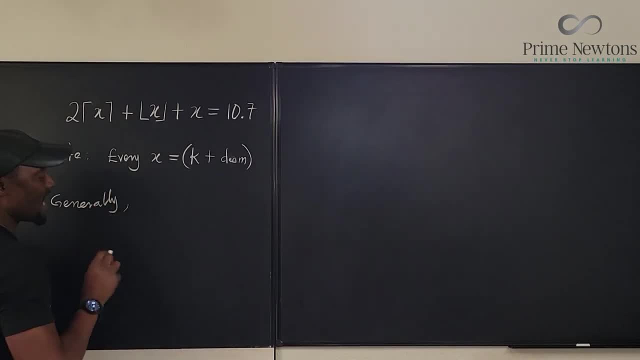 and that's what's going to help us answer the question. the ceiling of x is equal to k plus 1.. What is this k? again? It's this guy, Always, Always. And the floor of x Is k For all x. 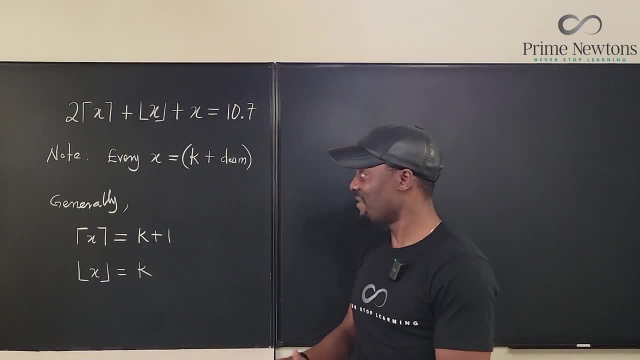 Okay, So the floor of x is k, The ceiling of x is k plus 1.. Okay, Unless. So watch this. Unless, k is an integer. So here we're saying k is not an integer, because if k is an integer, it is its own ceiling. 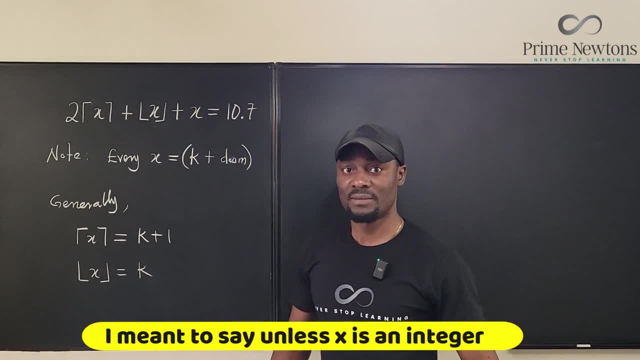 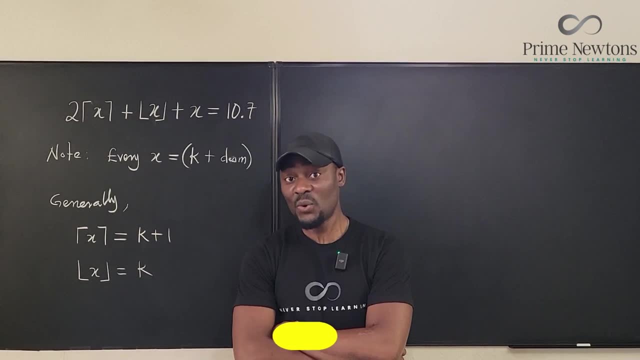 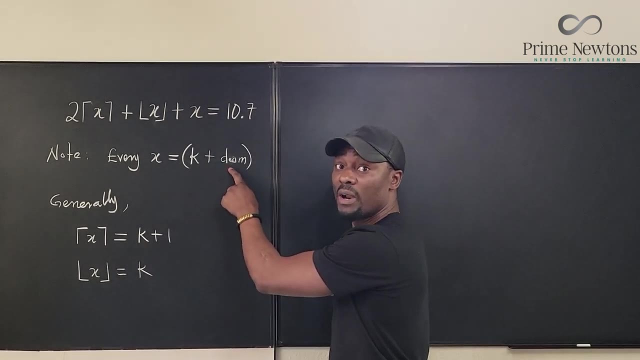 and it is its own floor. So, for example, the number 7,, the ceiling of 7, is 7.. The floor of 7 is 7.. Okay, So that's it. So the decimal part has to exist. 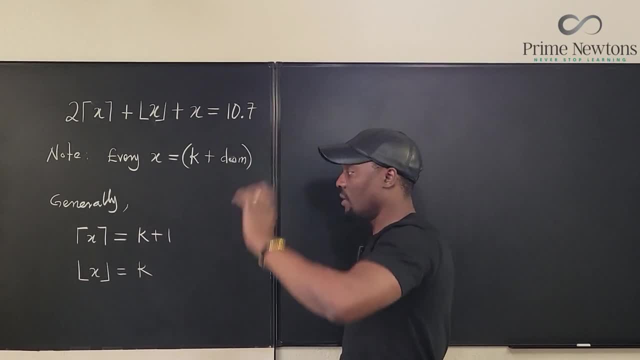 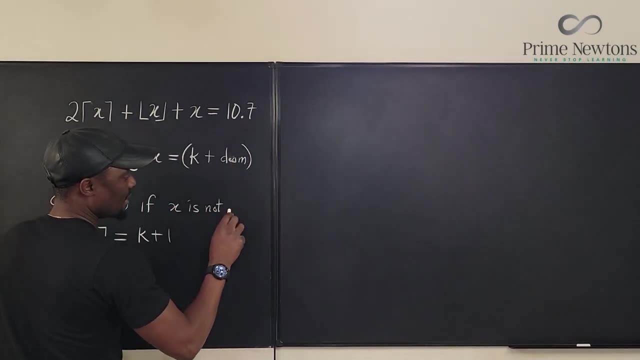 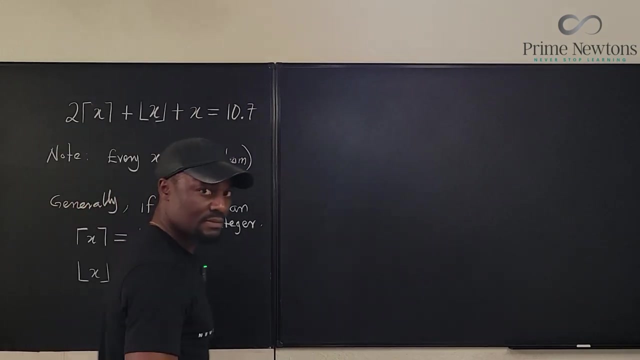 It cannot be 0 for it to be rounded up. Okay. So now we're saying, generally, if x is not an integer, let's write it here. then this is always true. Okay, If x is not an integer, this is always true. 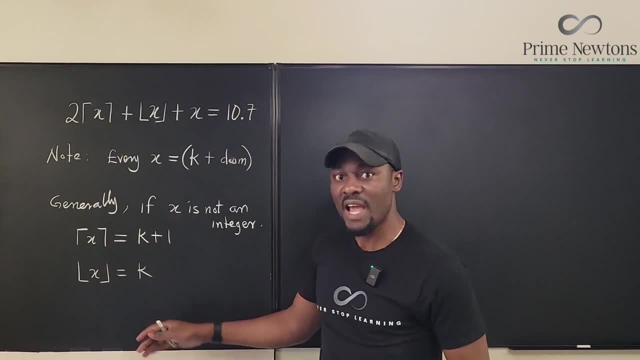 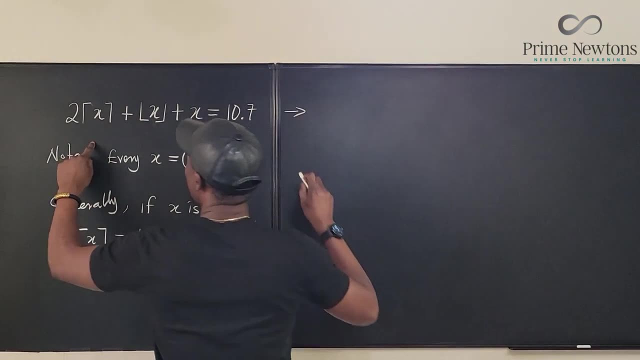 The ceiling of x is k plus 1.. The floor of x is k. With this explanation, just go here and solve it So we can say that this can be written as 2 times the ceiling of x, which is k plus 1.. 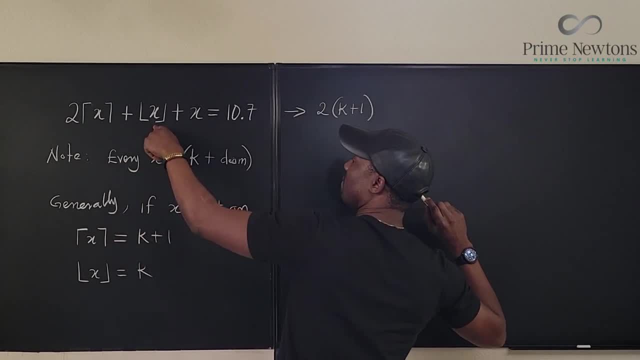 Plus what's this? The floor of x, which is equal to the floor of x, is just k Plus what did we say x is? We said x is k plus some decimal Right, So it's going to be k plus. 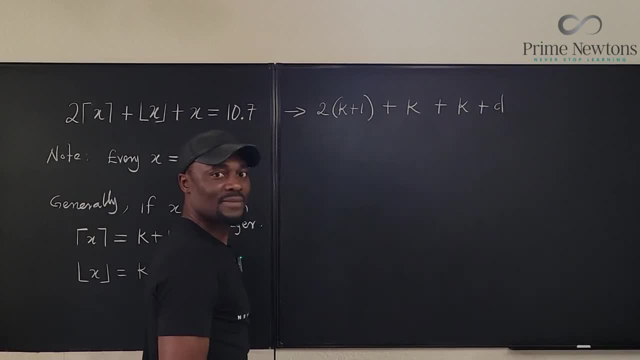 Now this decimal. let's call it d, And our answer is going to be 10.7.. So if we simplify this side, what do we have? We have 2k plus 2 plus k. Oh, this is. 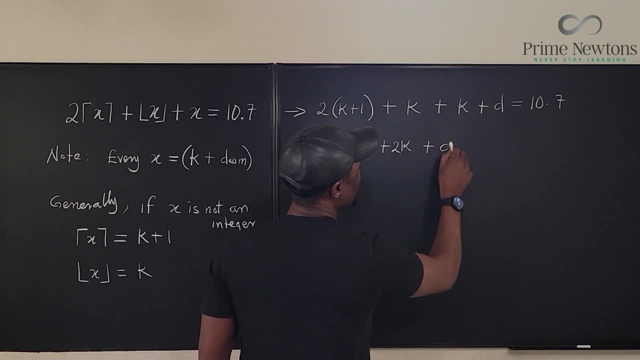 This is 2k again, Plus d equals. I'm going to write this as 10 plus 0.7.. If we add all of these together, we're going to get 4k plus 2 plus d. the decimal part equals 10 plus 0.7.. 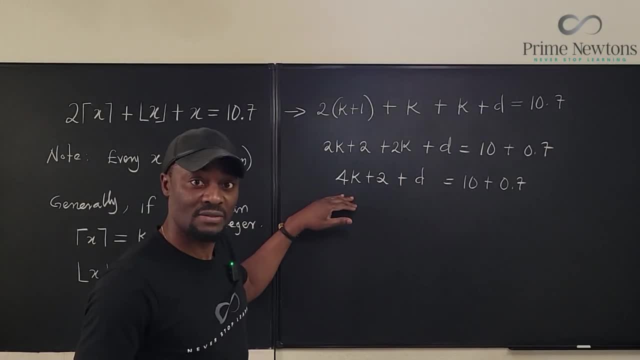 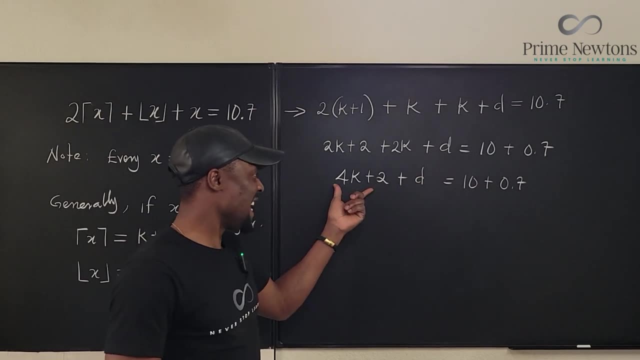 So, as you can see, there is only one decimal part on the left, There's only one decimal part on the right. So this decimal part must be this decimal part And this integer part, because the sum of integers is always an integer. 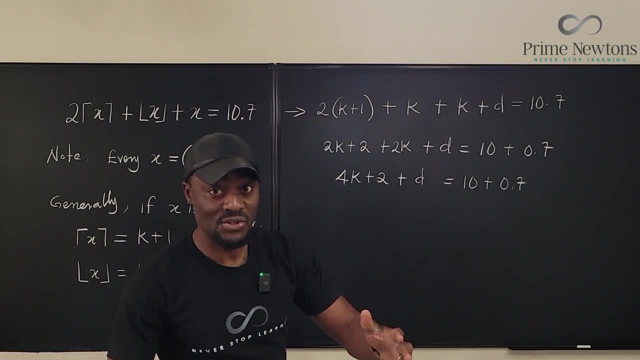 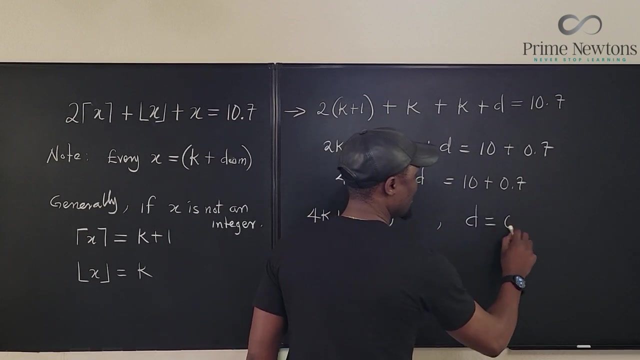 Okay, Remember that The sum of two integers is an integer. It cannot suddenly generate a decimal. So we're going to say 4k plus 2 is equal to 10.. And d is equal to 0.7.. So let's solve this.